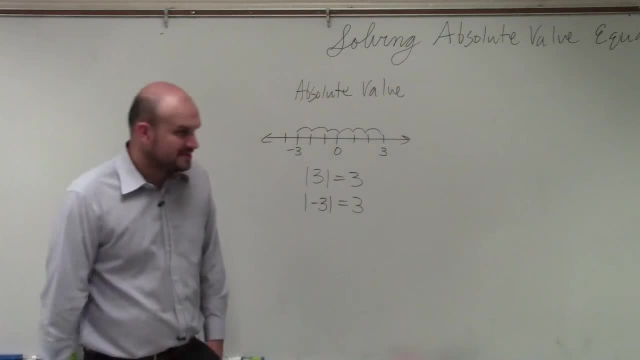 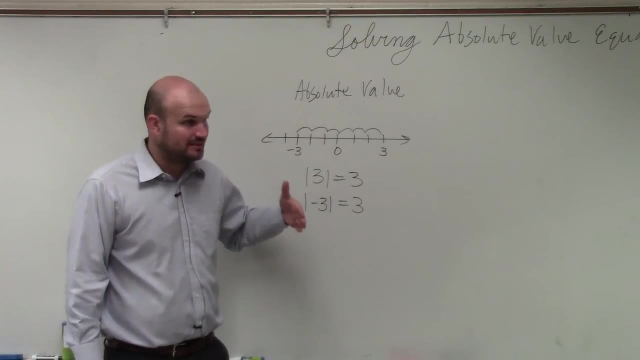 I didn't write that in there. So a couple of things that I want you guys to understand. First of all, the absolute value symbols represent absolute distance. They do not represent grouping symbols. They are not like parentheses Or like what do you call it? 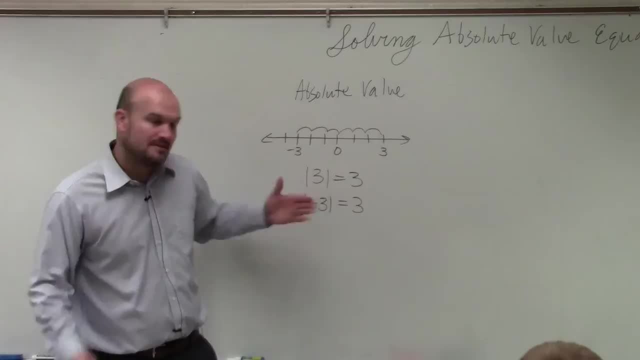 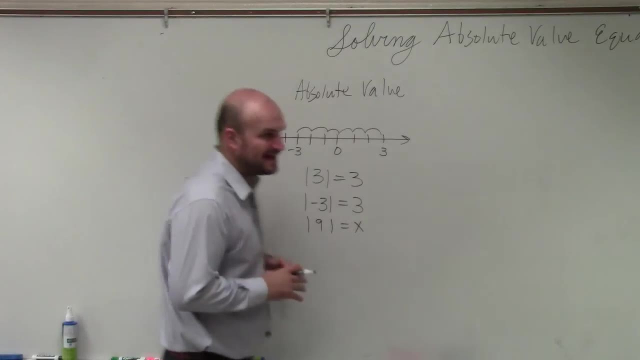 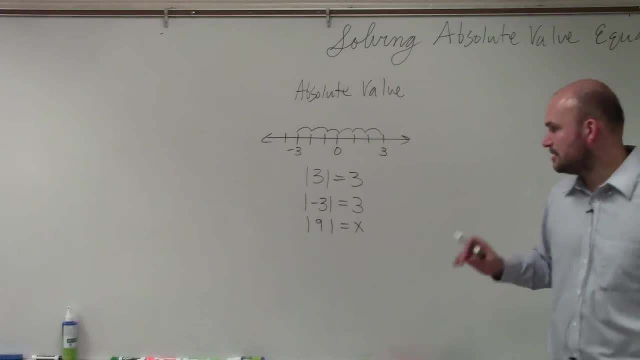 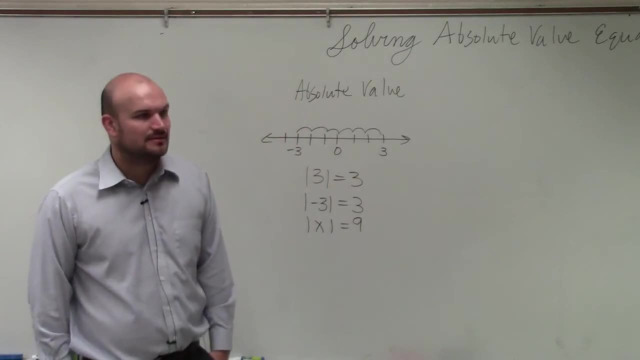 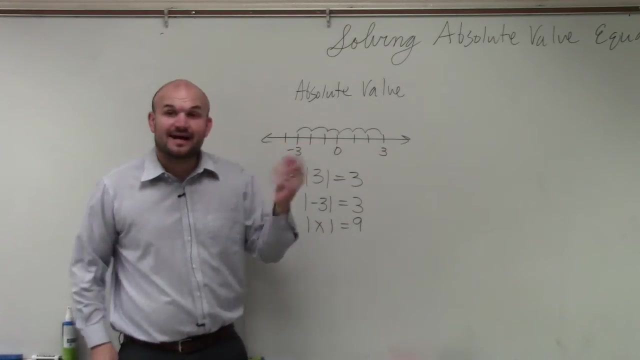 right. what could the values? um, no, whether wrote it wrong. what if the absolute value of X is equal to 9? what could my values of X be for me to equal 9? yes, I could have an x equals 9, right, because absolute value of 9, we know, is: 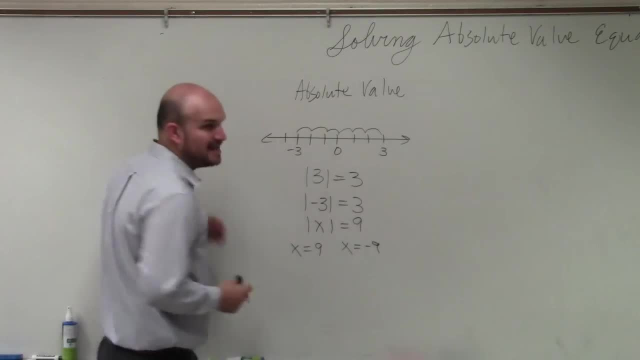 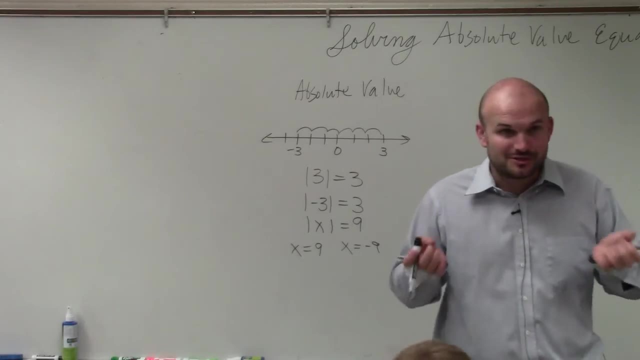 9, and I could also have X is equal to a negative 9. right, that very good. so there's something very, very important I need you guys to make sure you have, and if you need to write down, write down when we're looking for the absolute. 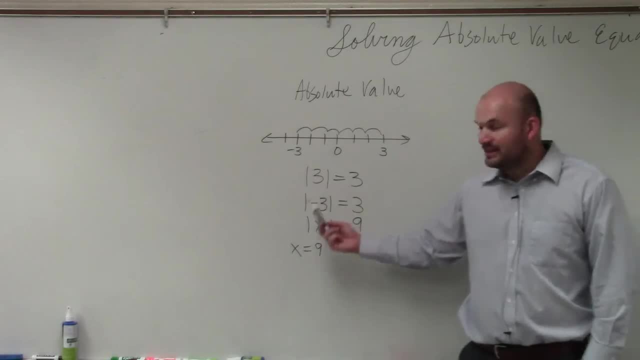 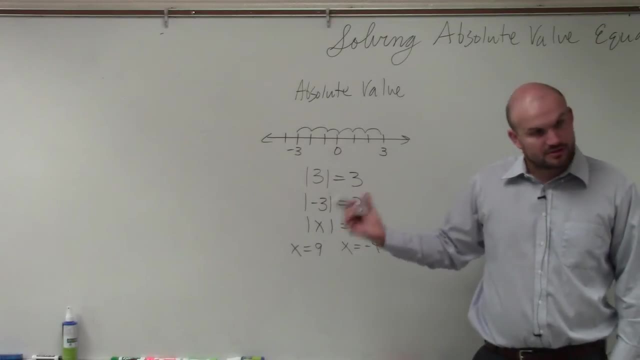 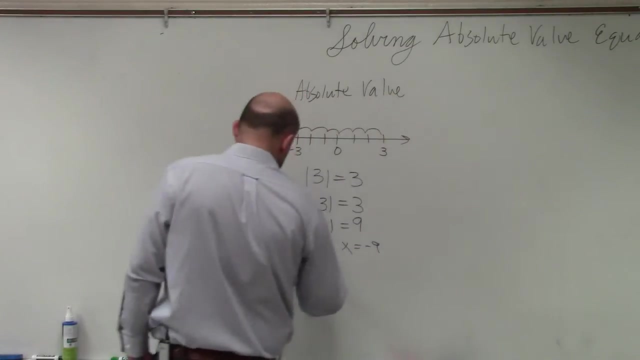 value. we're looking for two cases: when the quantity inside the absolute value is positive and when the quantity is negative. right, There's two cases: the positive and the negative of the quantity inside the absolute value, And then the last one we'll need to discuss before we get into a problem. 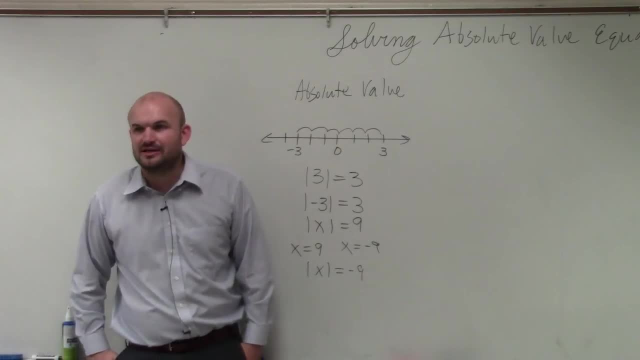 What about the absolute value of a negative? Can we have the absolute value be negative? Well, think, yes, Right, exactly, You can go negative direction. right, You can go in the positive direction, You can go in the opposite direction would be the negative direction. 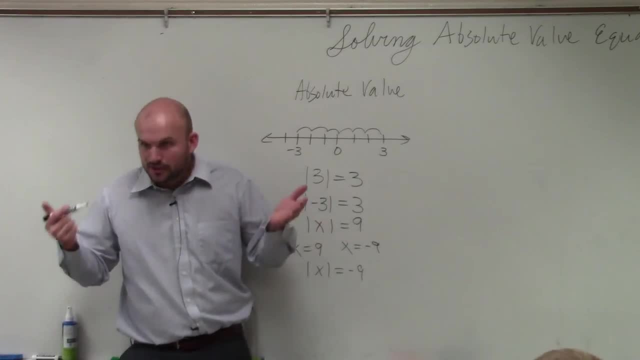 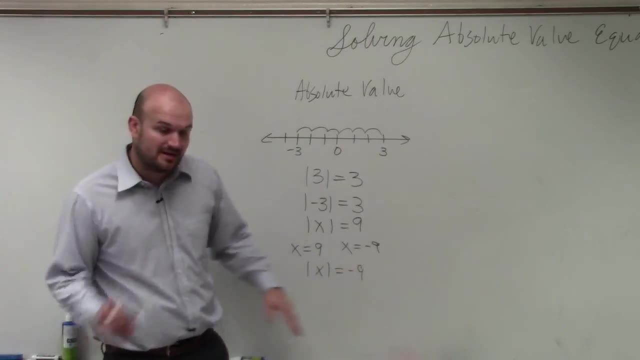 But you can't. you always go a positive distance. No matter what direction you go, you still went somewhere right. So if you have any time, you have an absolute value equal to a negative number. we call that no solution. All right, 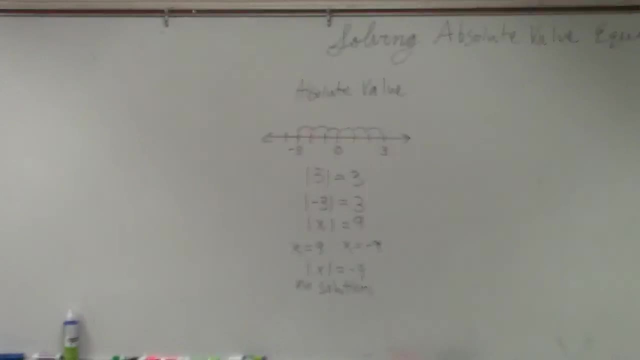 Okay, So now let's get into the fun stuff.